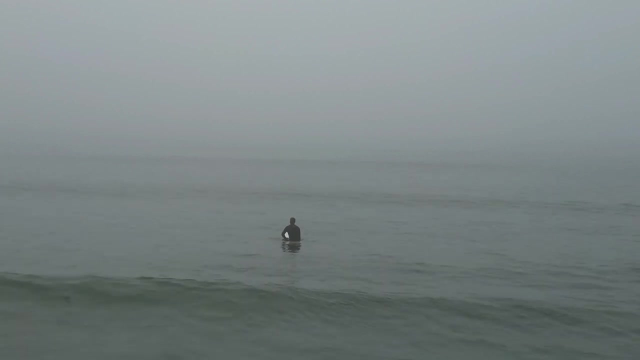 for is a distinct dark line, so you want to identify this as quickly as possible. the closer it gets to you, the bigger and darker the line will get. so what it is? because the tall waves are casting a shadow on themselves, where a flat wave has light reflecting off them, right. so it's. 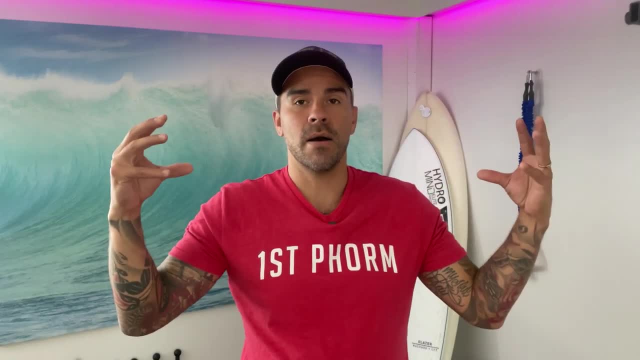 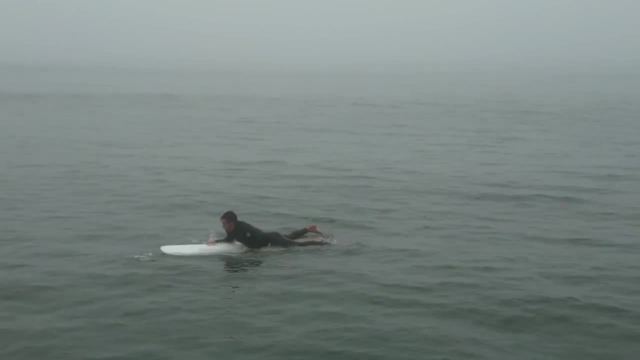 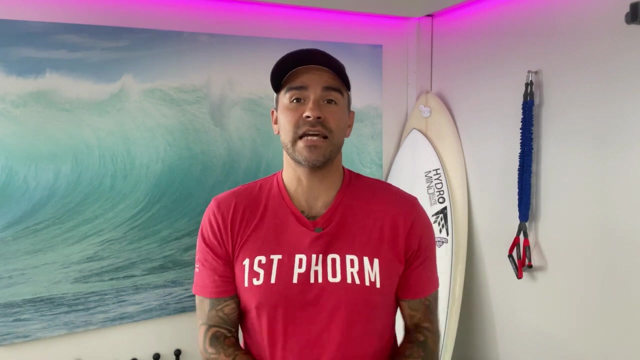 very, very distinct. so the darker the line, the bigger, um, taller the wave and it really really stands out against the small waves of the flat ones. So you can see the sets coming. you want to identify this as early as possible. so that's wave height, looking for that distinct black line. Number two: you need to identify the peak, so that's the. 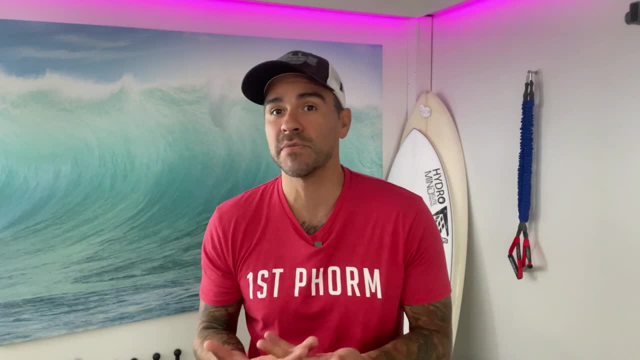 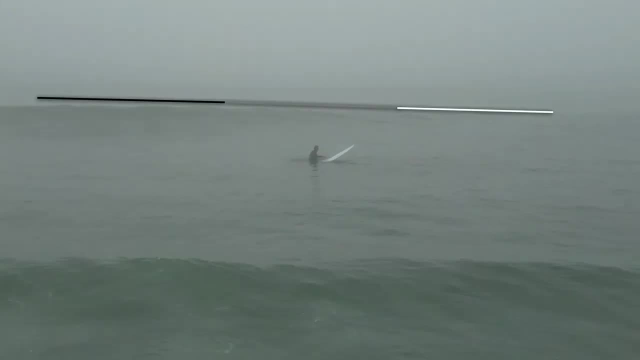 tallest part of the wave and again, because it's reflective, this becomes fairly simple. you see a distinct black line, or the tallest part of the wave, and it starts to fade off into more light because it's getting less and less steep. then that would be the peak. so that's um. sometimes it's very. 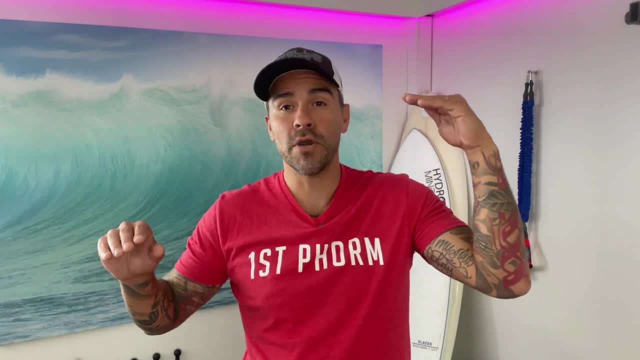 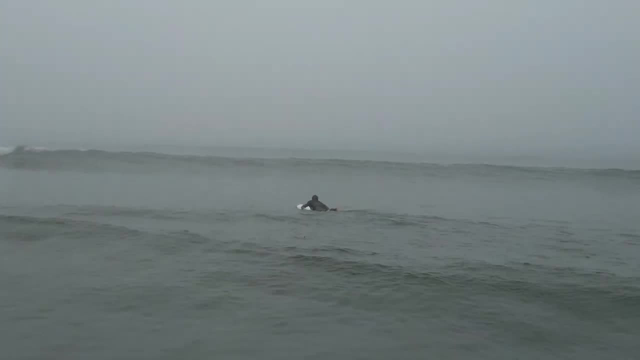 obvious, but often, quite often, it won't be obvious And it'll look like the black line is carried out over a long part of the waves. there's no obvious part. so it's really steep. it's really dark. it's really black, it's really flat. those waves are. 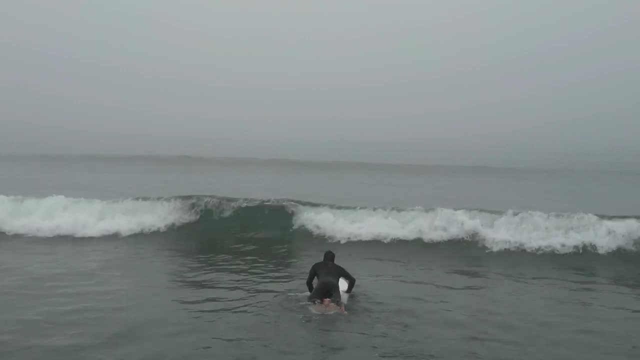 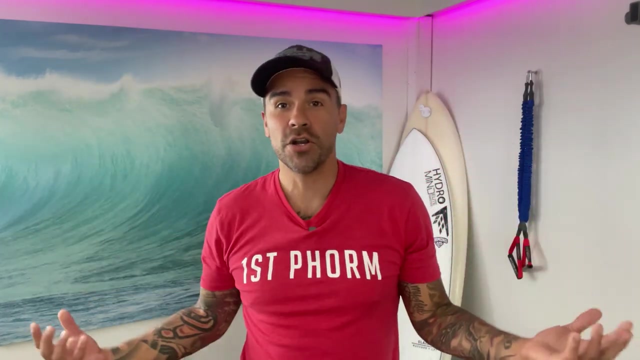 going to be closed out, so meaning the entire wave is going to fold over at once and it won't be going down the line like a nice ride. so if you take off on that wave, the entire wave will fold over and land on you, or you'll just get caught out in front of it and you'll be caught inside and the rest of 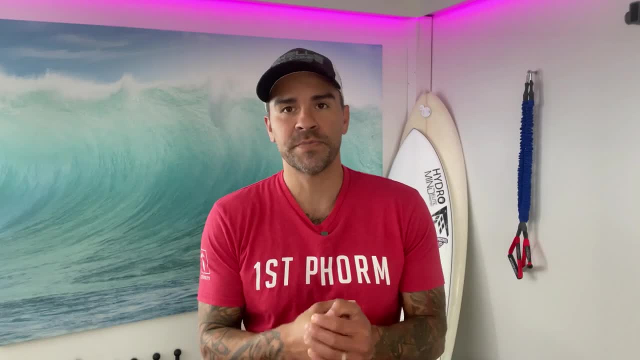 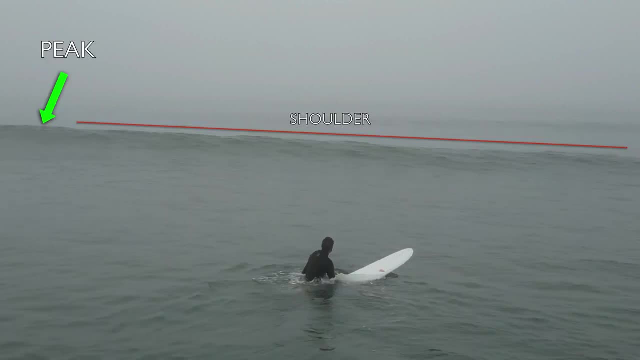 the waves are going to come and land on you, so you want to avoid those waves. Once you've identified the peak, the third part is going to be the peak, And this is a very important one that lots of people miss because they'll just go for any peak. 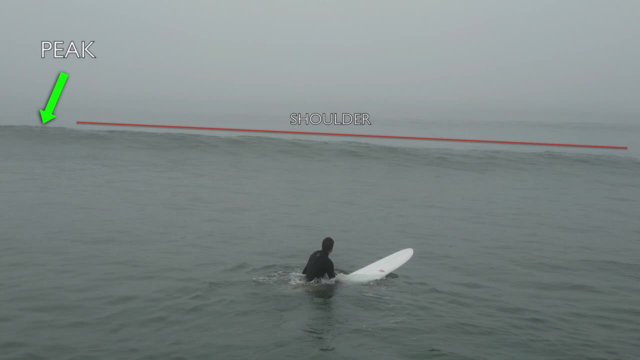 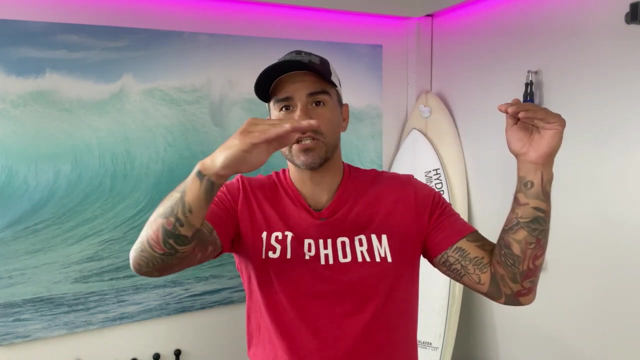 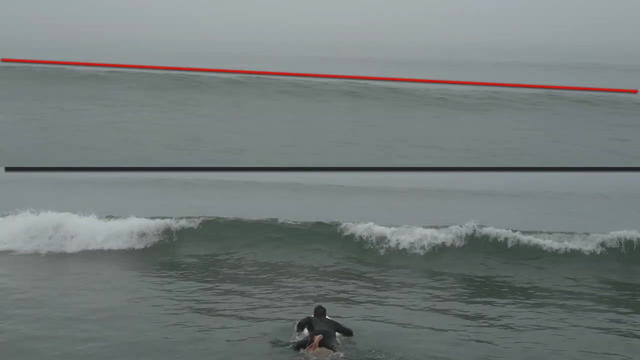 is the shoulder and really what the shoulder is, how much water is in that wave? so what you want to look for is a shoulder that is long and very gradual. this is where it gets tricky, because a closeout is tall all the way and a gradual shoulder that you want is slight, right. so 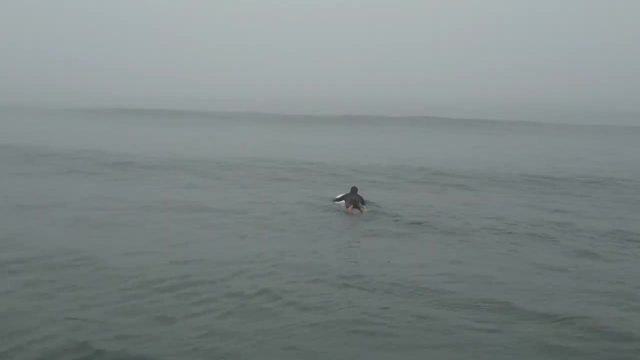 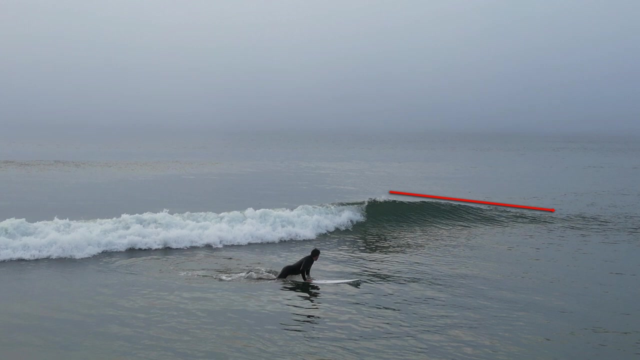 it's very, very slight. what you're looking for is that change of color with an obvious peak. the flip of that is a short shoulder, so it's very steep and very short and it tapers off into nothing. so that'll be a fast wave, but a short ride because there's not much water in it, there's not nothing. 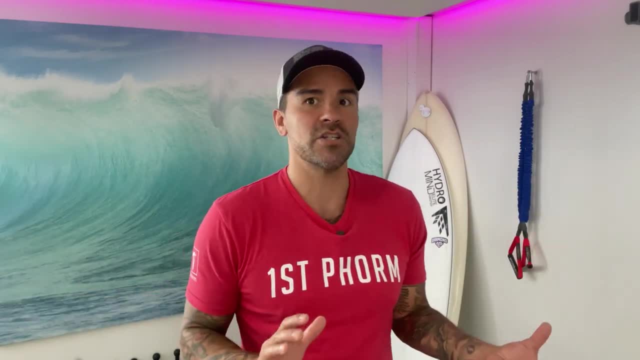 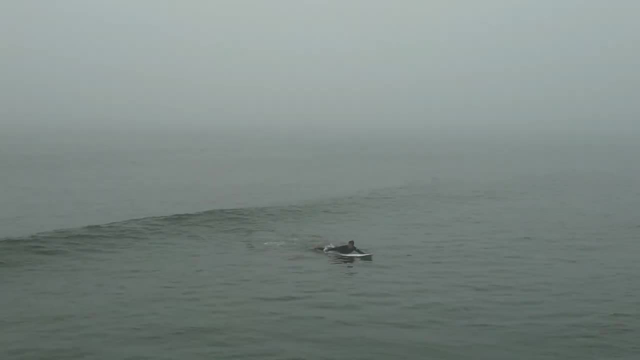 left for it to break. it'll break down to nothing and be gone. so you'll spend the energy for a very short ride, very often not worth it. so you want to find the tallest waves, the dark line, you want to find the obvious peak and you want to find the ones with the very long shoulders when you combine. 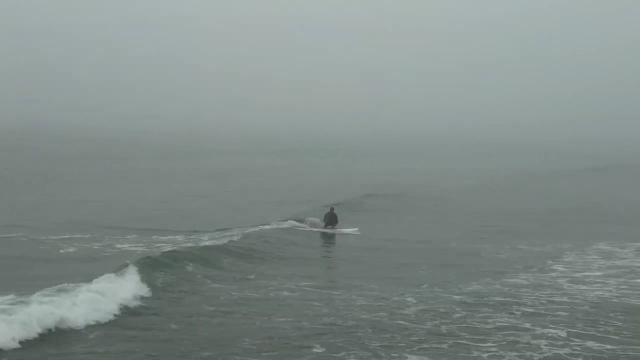 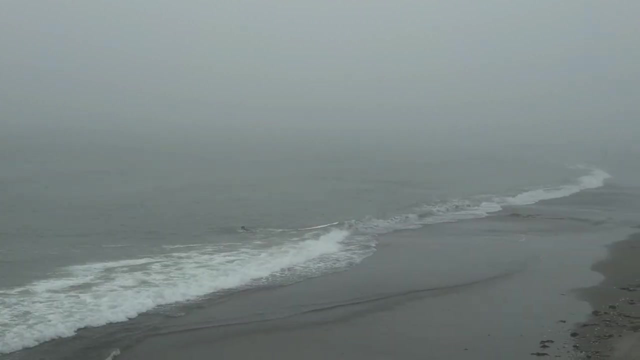 those three things, you'll have a long shoulder and you'll find the short shoulder and you'll find the long smooth ride, and you won't waste energy on those waves that you shouldn't be catching. so what i've given you is a three-step process, but really it's one step as you get good at this. 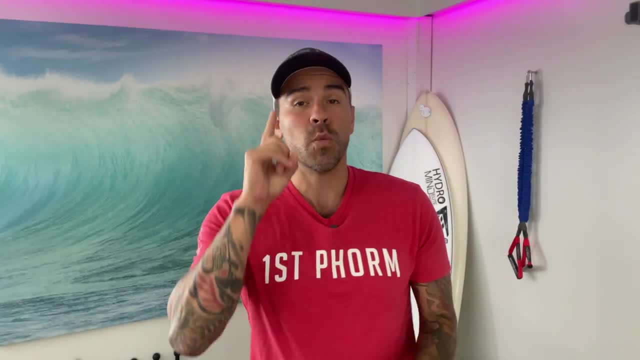 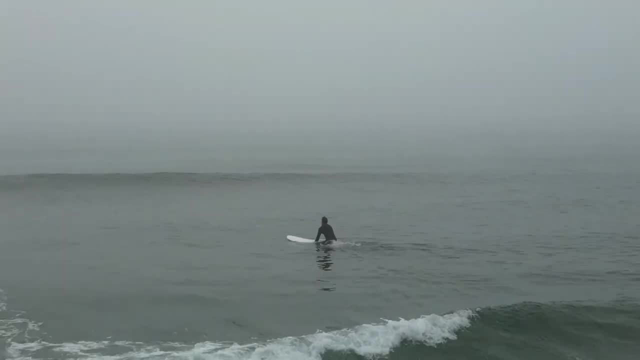 you should be able to determine if it's a good wave or a bad wave with one glance. and the real skill comes with identifying this as early as possible, because when you're looking out on the horizon, you start to see things like: is that a wave? is it a big one, is it not? the sooner you 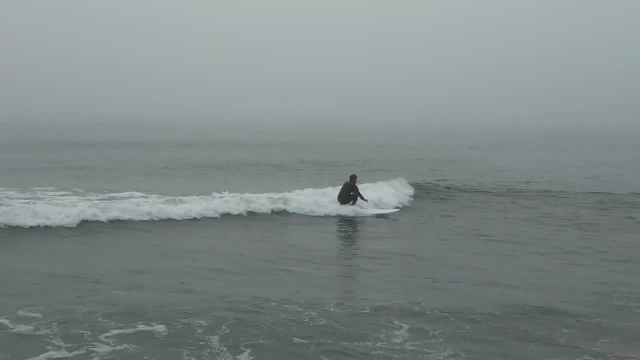 can tell the farther away that it is where you can determine this, the better off you are. you're going to be able to determine that, and you're going to be able to determine that the you can make a decision like: okay, the peak's over there, i got to move this way. it peaks over here. i. 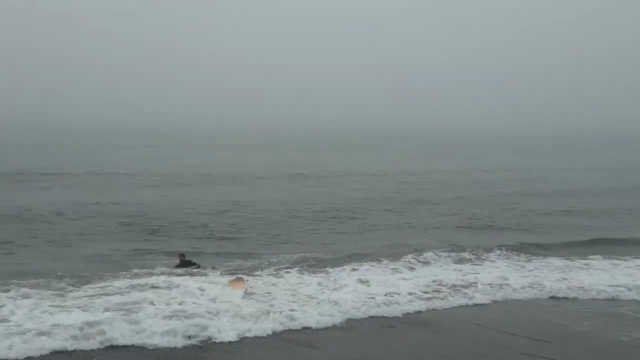 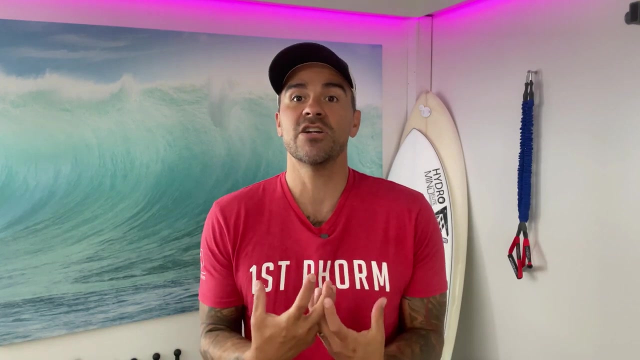 gotta move this way. it's not worth it. i'm not gonna waste energy. it's got a great shoulder. okay, i'm gonna attempt this wave. so the quicker you can make that decision, the better positioning you can be in and the less energy you can waste and you can save that energy, those bursts for the. 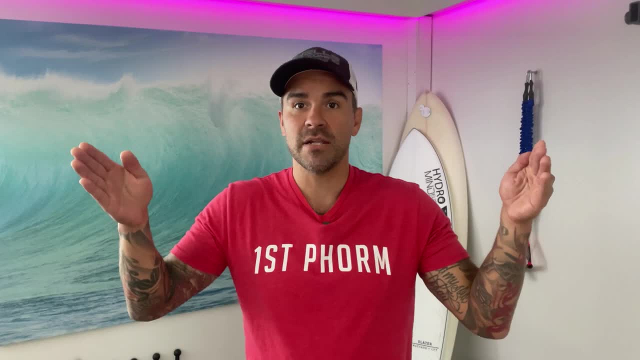 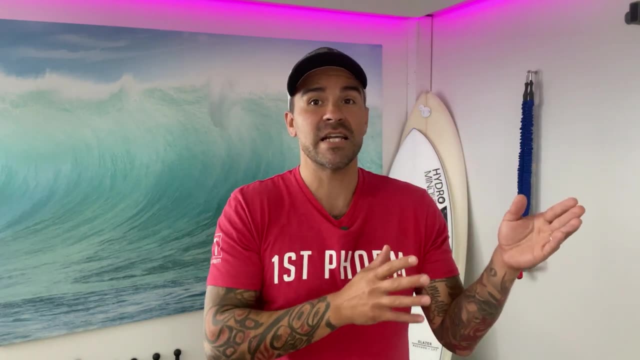 best waves because each session you have a limited amount of energy, like a battery, and if you're spending that on missed waves that means more frustration, last wave, less progression. so proper wave selection means you're spending your energy in a good way. that's moving forward and making sure. 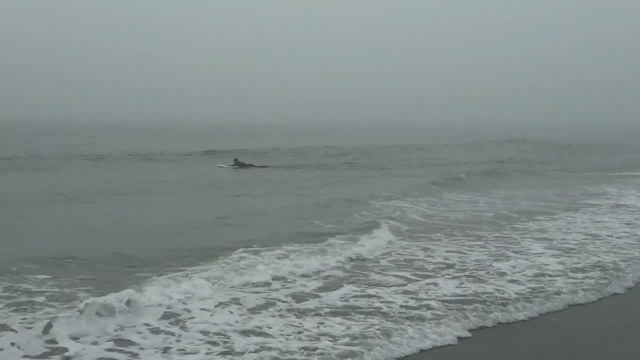 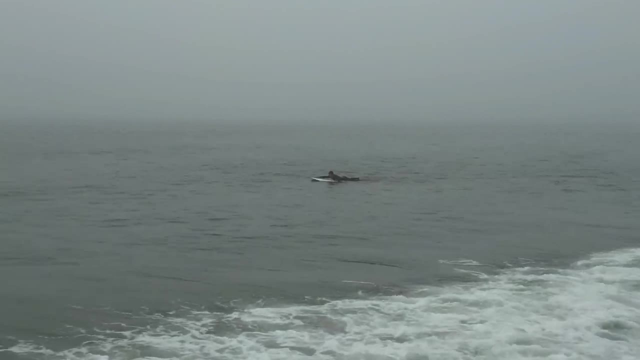 you're having a better, more fun time, and that's how you reliably do it. the coolest thing about this skill is it can be done from the beach. you don't have to be surfing, you can be out there testing yourself so you can see a wave. go through this process of reading it determine in your mind. 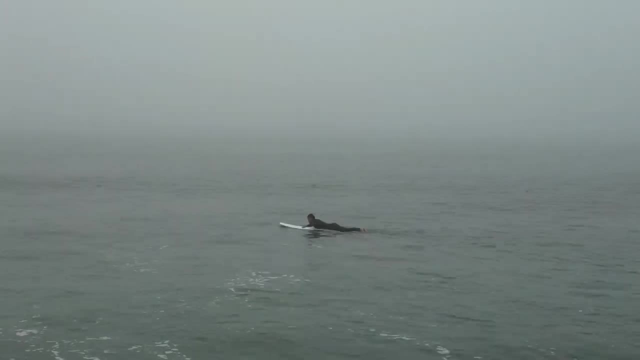 whether you would go for it or not and you can watch it play out in real time. be like, yeah, i would have went on that one, oh wait, it was a closeout, what did i miss? and be like: oh, that is a closeout, and you watch it how it folds over, right, so you know exactly how it works. 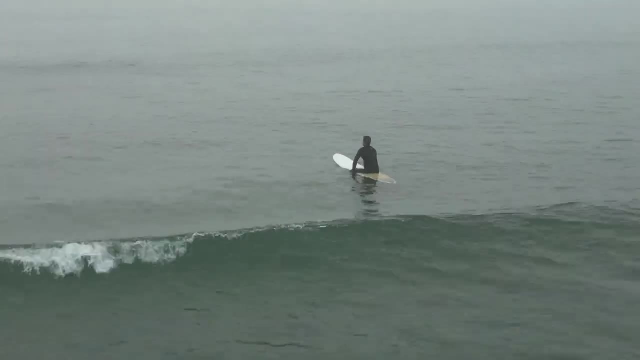 you can do it at every spot, before you paddle out and when you get in the water and you're up close and personal, you have a way better understanding of what this wave is going to do, how it reacts at certain spots, where you should sit, where you.